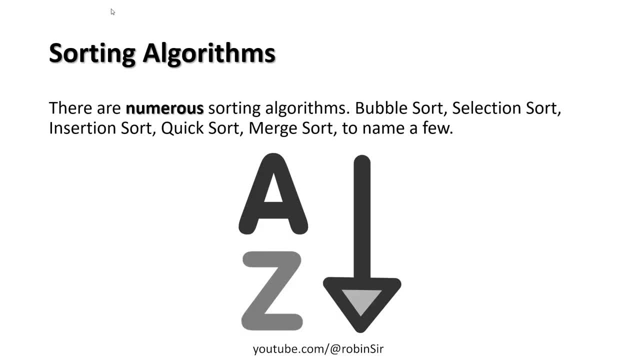 Now, here I have listed some sorting algorithms. There are many, many sorting algorithms: Bubble sort, selection sort, insertion sort, quick sort, merge sort are some of these sorting algorithms. Now, why am I listing all of these sorting algorithms? 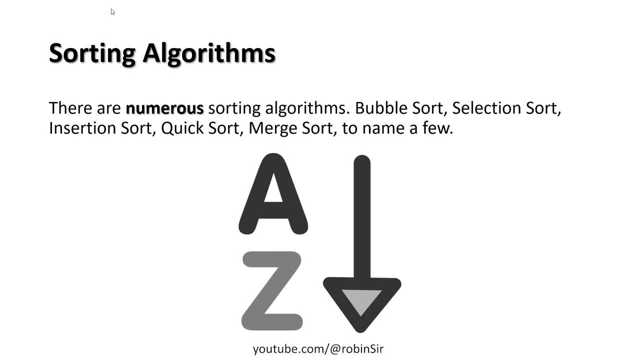 Because now one question arises: When there are so many sorting algorithms, how can I say which algorithm is better than the other? How can I compare two algorithms? So we want to compare two algorithms and say, okay, this algorithm is better for sorting because this algorithm is faster. 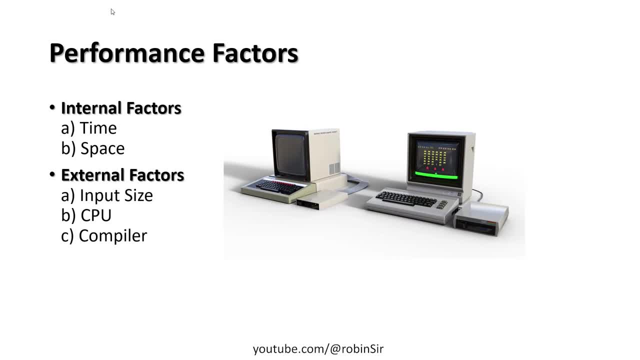 So to compare two algorithms or to measure the performance of any given algorithm, there are internal factors As well as external factors. Under internal factors we have time and space, Meaning how much time an algorithm takes to solve a given problem. 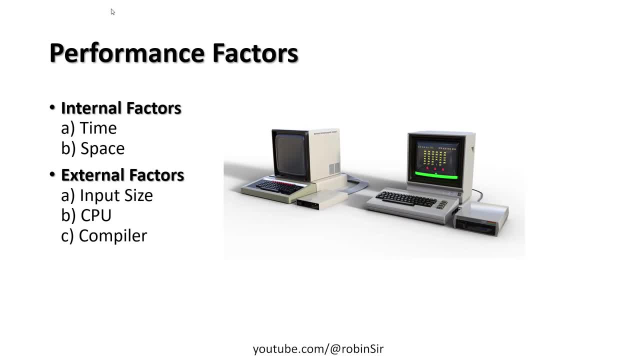 And space means how much memory the computer is taking to solve that problem. And there are some external factors also, like the input size. How much data are we working with? Is it just a number? Is it just a small set of data? 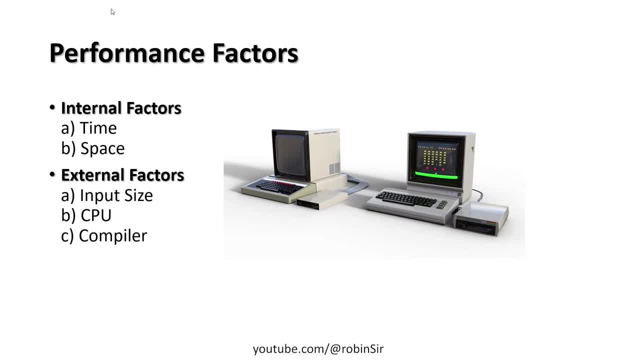 Or is it a huge amount of data, Let's say millions or billions of data? Another external factor is the CPU speed or the CPU power. If you have a faster CPU, the performance will improve, to some extent Also the compiler. If the compiler is efficient, then also the performance of a program can improve. 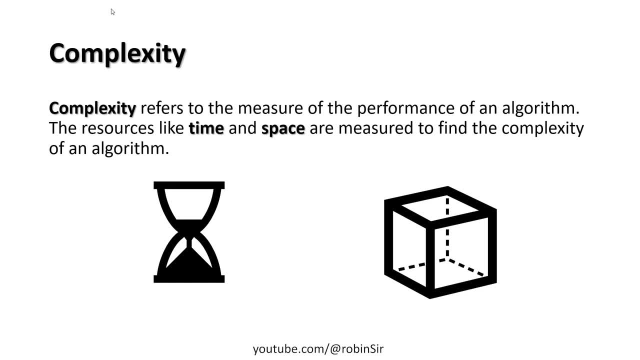 So we saw that the title of the chapter is computational complexity, So computational means. here we are doing some kind of computation, We are solving a problem at hand, Whereas complexity means measurement- How fast or how quickly the computer is solving that problem. 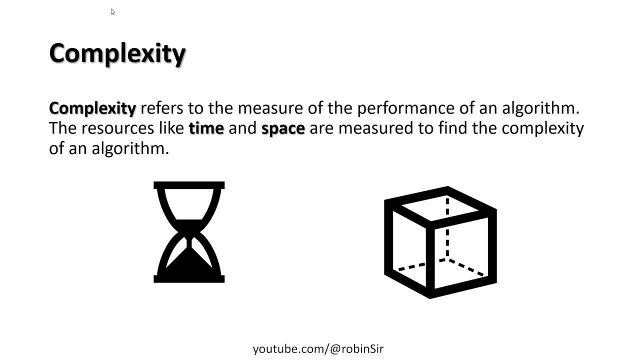 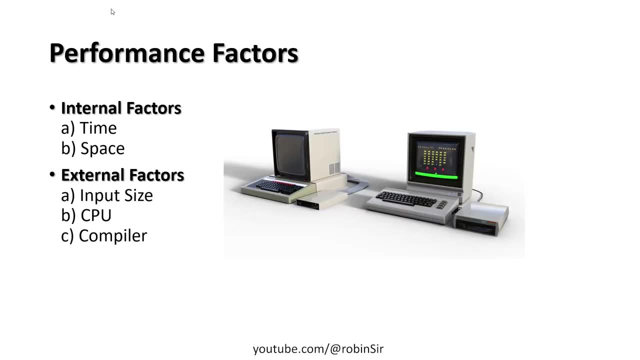 So complexity refers to the measure of the performance of an algorithm. The resources, like the time and space, are measured to find the complexity of an algorithm. So you saw in the previous slide that we have both internal factors as well as external factors. 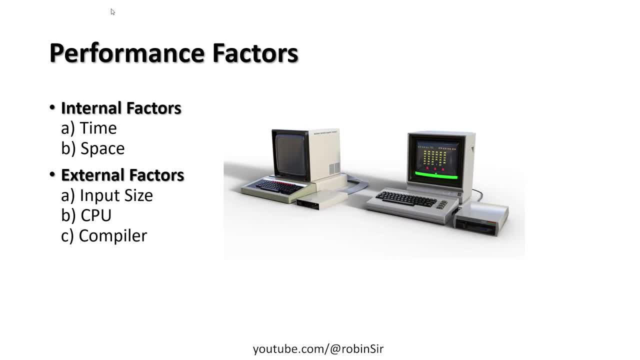 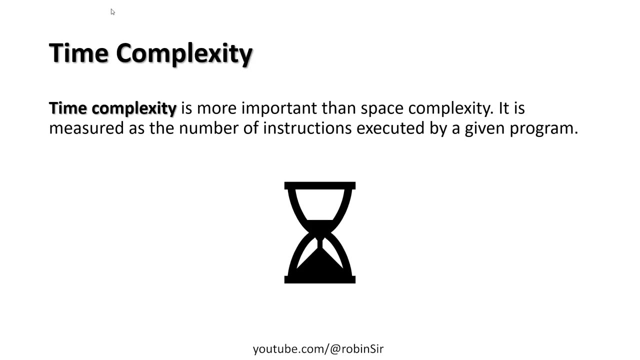 But internal factors are considered to be much more important than the external factors, And out of time and space, time is considered to be more important. So what is exactly this time complexity? So time complexity is measured as the number of instructions executed by a given program. 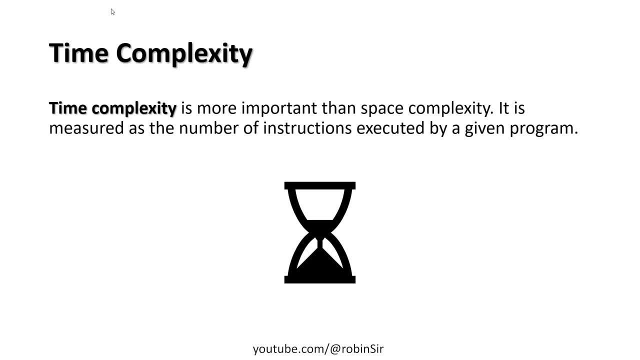 When we hear time complexity it sounds like we have to measure time in seconds or milliseconds. maybe Time complexity actually means the number of instructions executed. So if a program takes seven steps to solve a given problem, so that's the time complexity of that program. 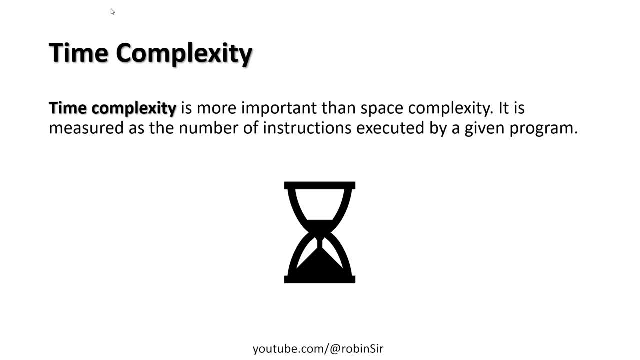 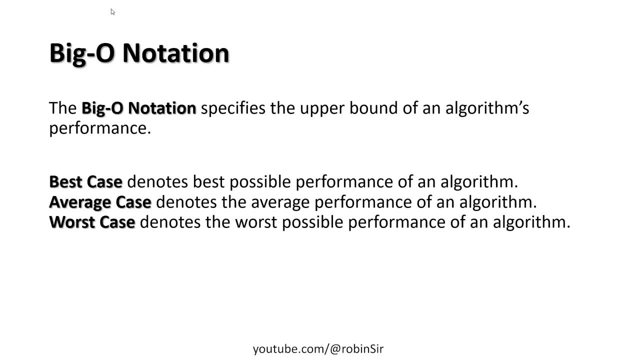 It's actually the number of steps taken by that program to solve that given problem, And we will be using Big O notation to measure the performance of an algorithm. Now, what is Big O notation? So Big O notation is a function that tells us about the 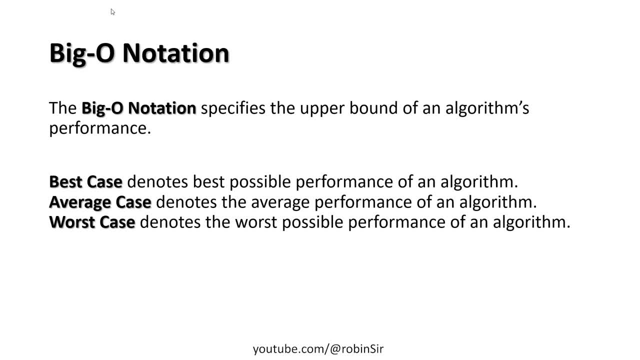 what is the worst possible performance of an algorithm. So an algorithm can have best case, average case or worst case. Best case means in what situation an algorithm can give optimum performance. Average case means when you are running the same program several times and you find out the average performance. 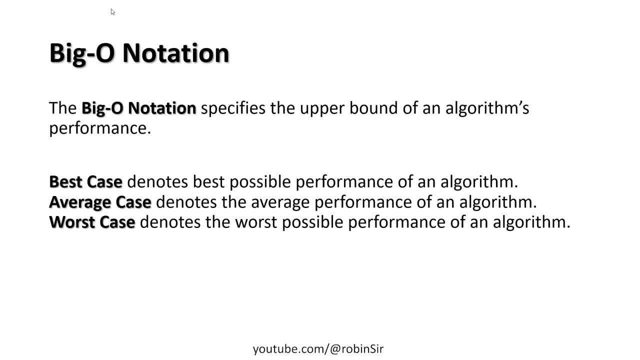 that actually indicates the average case, And the worst possible performance is when you are running the same program several times and you find out the average performance. worst case means what could be the worst situation for that particular program and how is it going to perform during that worst situation. So we will try to understand this with an example. 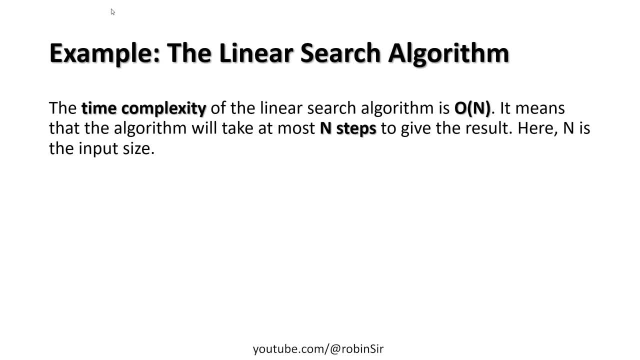 So we have taken the linear search algorithm. The time complexity of linear search algorithm is big O, n. Now what does it mean? It means that the algorithm will take at most n steps to give the result, not more than that. And n is the input size. So suppose you have an array of size n. 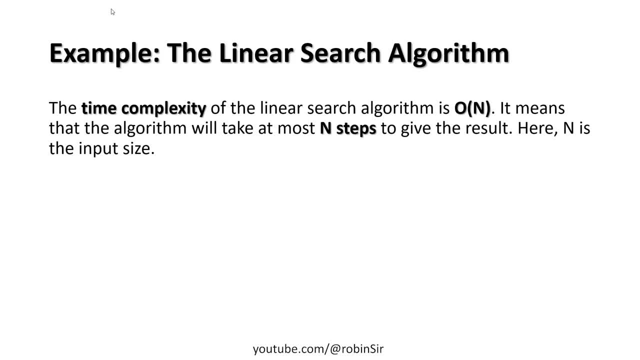 So in the worst case, what might happen in linear search? In the worst case, the element that you are searching for might not be present in the array. So that is an example of the worst case. In such a case the program will go through all the elements one by one, from starting till the end. 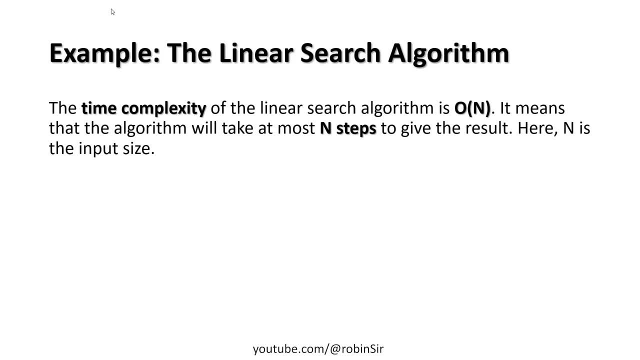 and then it will realize that the element that you are searching for is not present. So that is why we can say it takes n steps maximum to solve that problem. So if your array has size 100, it can take roughly 100 steps to give the result. 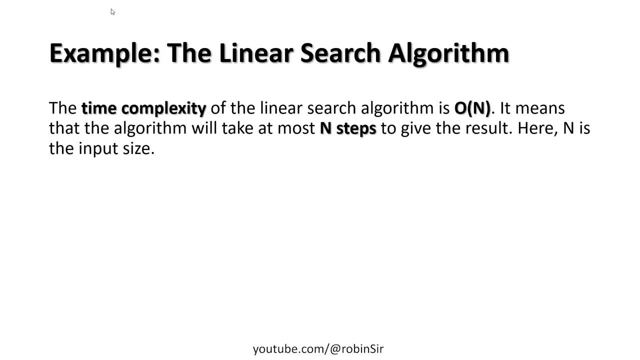 What could be the worst case? In such a case, the program will go through all the elements one by one, from starting till the end, and then it will realize that the element that you are searching for is the best case, When the element that you are searching for is present at the very first index. 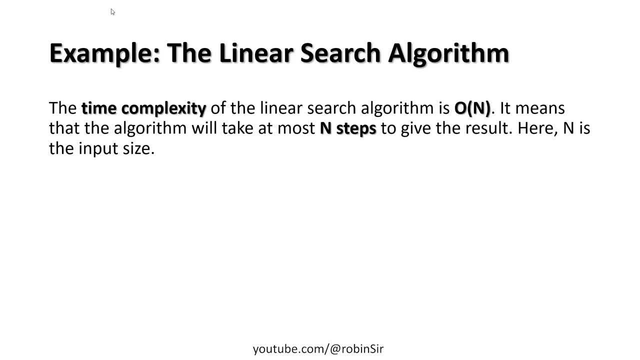 that is, index 0. So the very first element. you compare and you found that element right there. That is an example of the best case, An average case. So randomly you are searching for elements, You run the program several times, You find out the time, complexity. 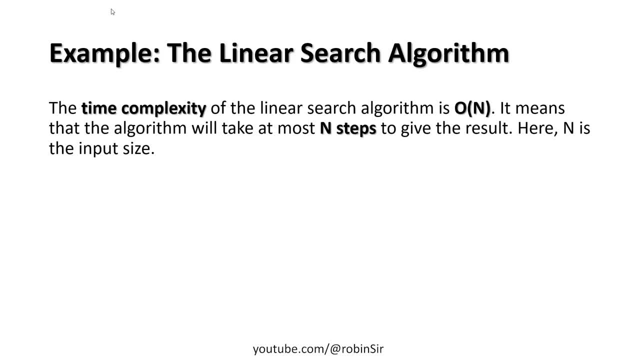 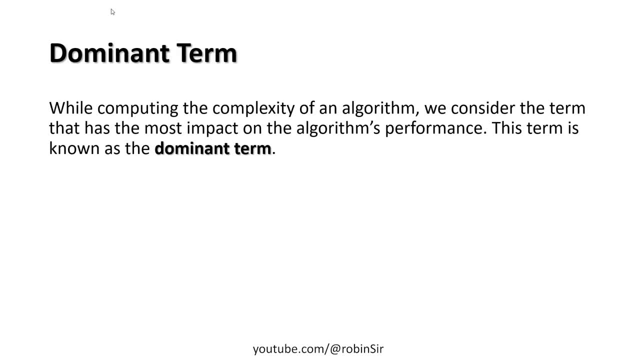 each instance and then you find out the average. that's the average case. now, when we are finding the time complexity or space complexity, we have to look for the dominant term. what is the dominant term? so, while computing the complexity of an algorithm, we consider the term that has the most impact on the algorithms. 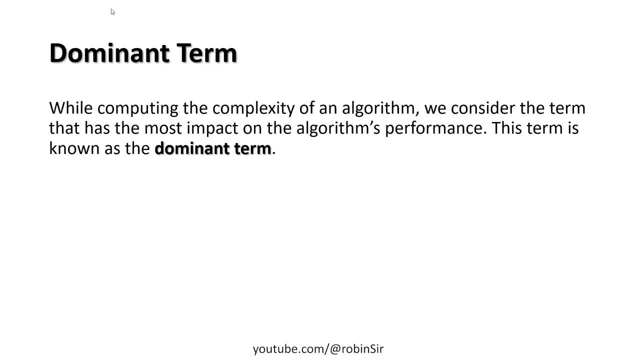 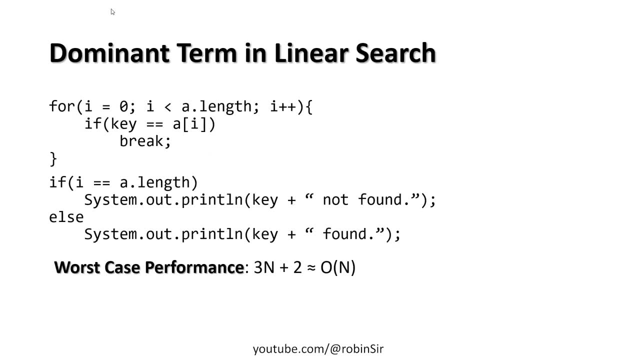 performance. this term is known as the dominant term. again, we'll try to understand this with an example. so again, I have taken linear search over here and you can see that the loop is running n times, depending on the size of the array, and in each iteration three things are happening: the condition is checked. 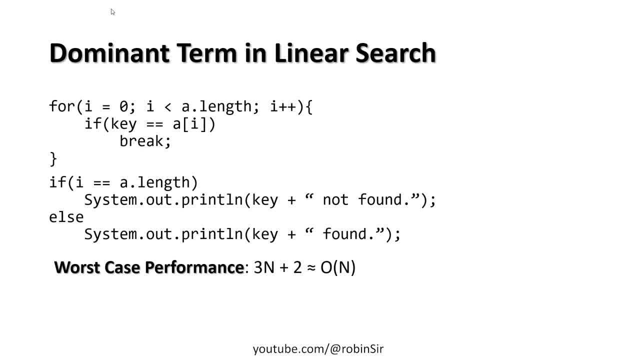 whether i is less than a dot length or not. if the condition is true, we enter and we check the condition if key is equal to a of i or not. if it's true, then break will execute, but if it's not true, then i plus plus, which is the third statement. so i 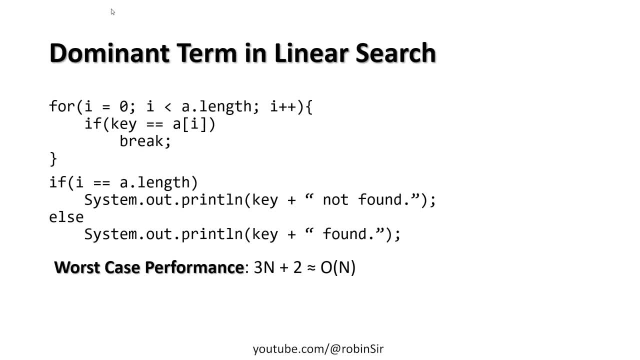 plus, plus will execute. so that's why, in the worst case performance, here I have written 3n. so you can see, here I have written 3n because this loop is running n times, where n is the size of the array and three tasks are being repeated. this for loop, condition if condition and i plus. 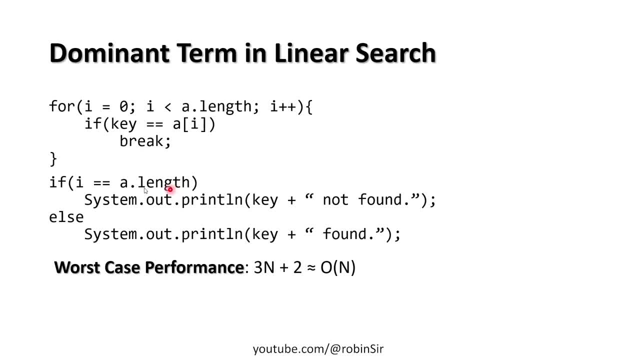 plus, so three times in once. the loop ends. then this: if condition is being checked, if the condition is true, the first statement executes. otherwise the second statement executes. so condition and the statement, two tasks. so that's why plus two. and when we look at this expression we see that this part 3 n is. 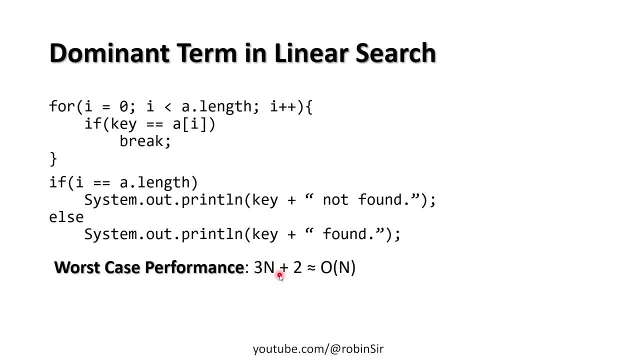 the dominant term, because when n will be huge in size, when n is very big plus 2, will be trivial, it will have you know. if it's going to be less than a dot length, it will be trivial, it will have you know. if it's, it will be negligible. so that's why 3n is dominant. and again, when we look at 3n, 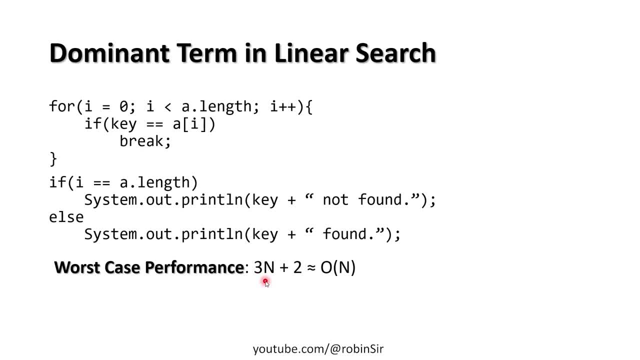 when n is very big, 3 times n will not make much of a difference, so 3 is also being ignored, and so we can say that the worst case of the linear search algorithm is big O of n. let's take another example: time complexity of bubble sort. 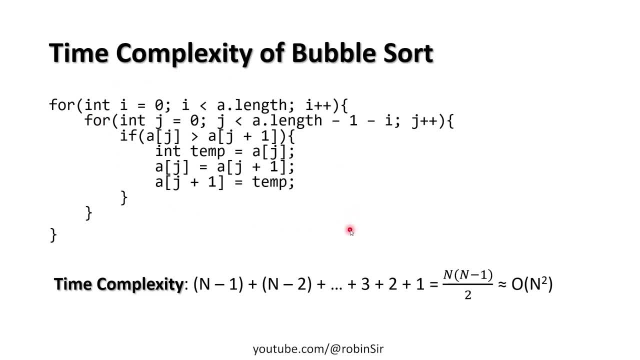 now we know that for bubble sort we run a nested loop, so this inner loop is more or less, you can say, running n times. so firstly the inner loop runs n minus 1 times, then n minus 2 times, n minus 3 times until 1 time, and we know that the sum of this series 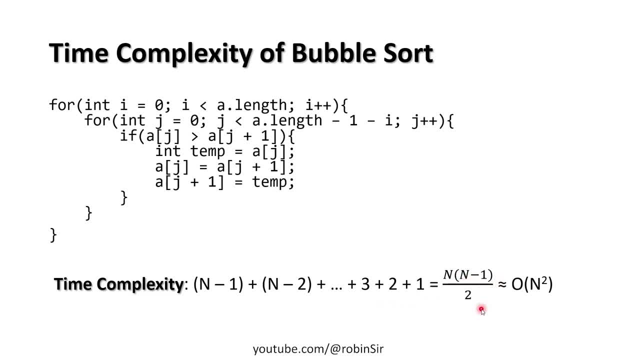 is n into n minus 1 by 2. so n minus 1 is almost the same as n. so we can say n squared and divide by 2 doesn't make much of a difference. so we can say n squared is the dominant term here. so we can say the time complexity of bubble sort is big O n squared. so if we have 10 elements,